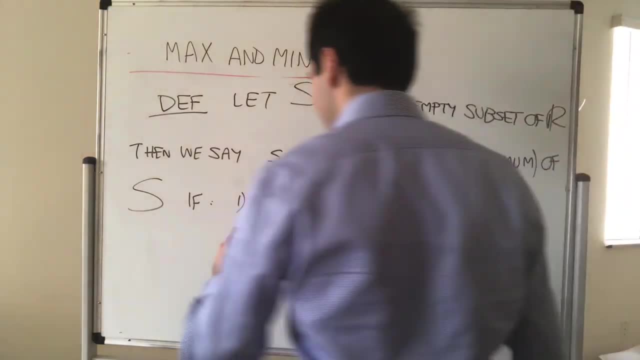 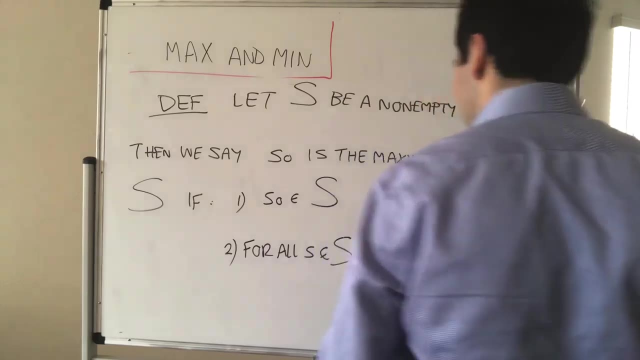 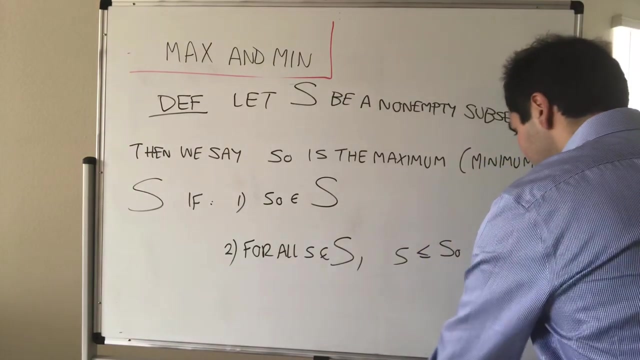 you're better than any other student in this class. So in other words, for all S, S and S we have, that S is, in other words, any other student is inferior to you. So S is less than or equal to S naught. 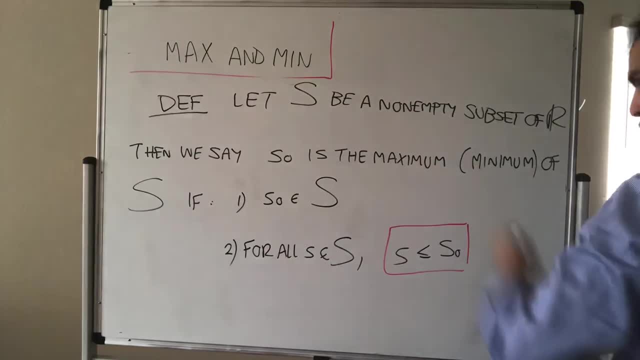 That's for maximum. For minimum, it means you're inferior to everyone else. So in other words, S is greater or equal to S naught. So S is less than or equal to S naught. So let me just illustrate this with a picture. 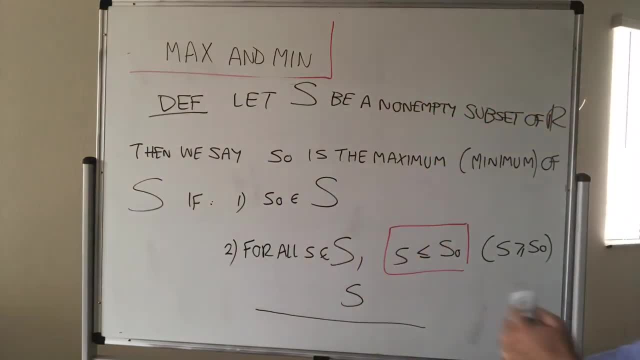 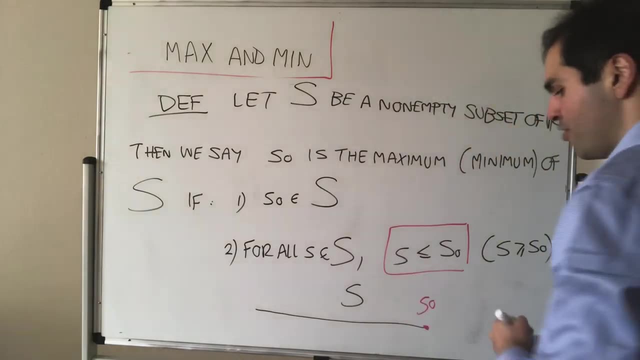 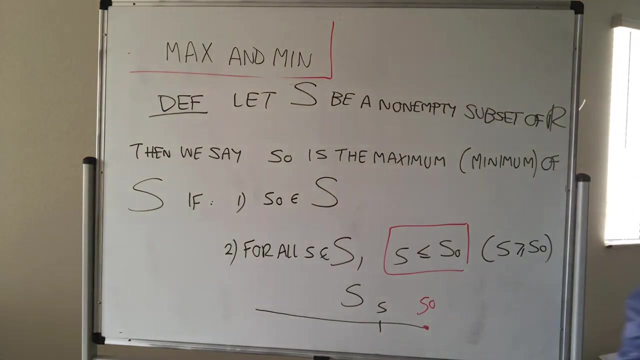 So suppose this is your set S Again, what does that mean for S naught to be the largest value? It means that whenever you take any other value of S, it has to be less than or equal to S naught. And for the rest of today. 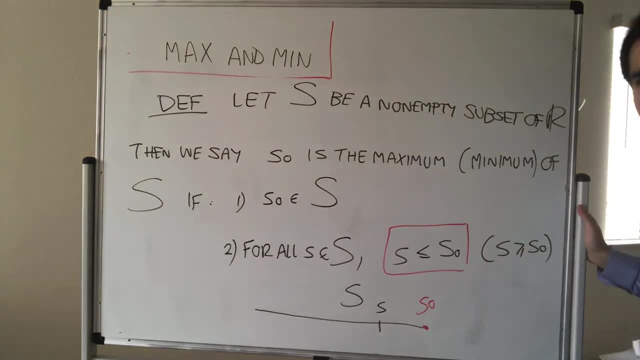 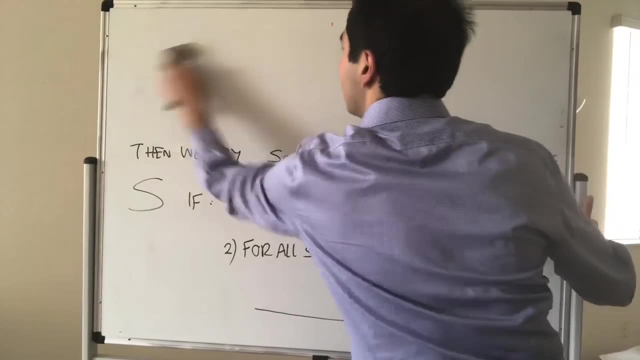 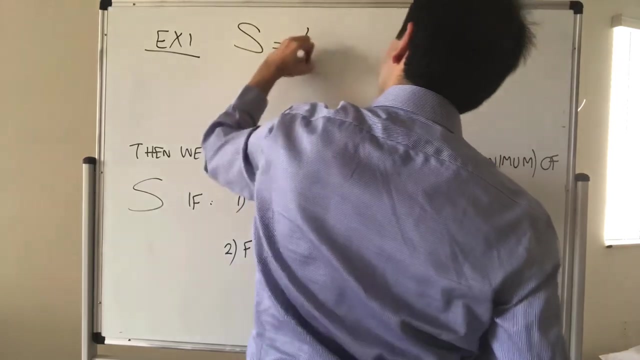 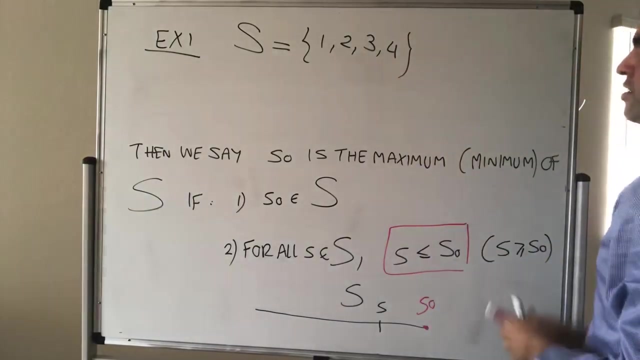 we'll just do a bunch of examples, but again, very important definition. So for instance: well, take S to be the set one, two, three, four. Then well, what is the largest element of that set? Well, it's four. 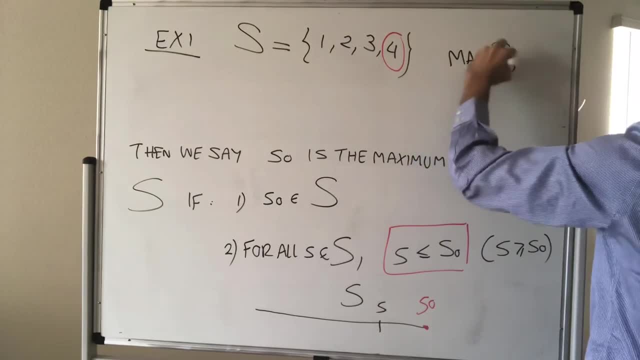 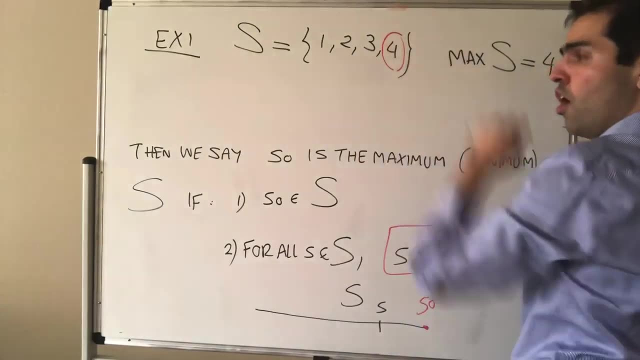 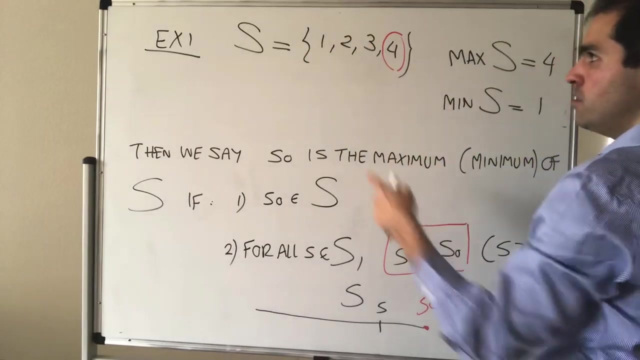 Then the maximum of S is four because, look, four is in your set and also four is larger than all the other values in your set. And similarly, the minimum is just one, because one is in your set and one is smaller than all the other values in your set. 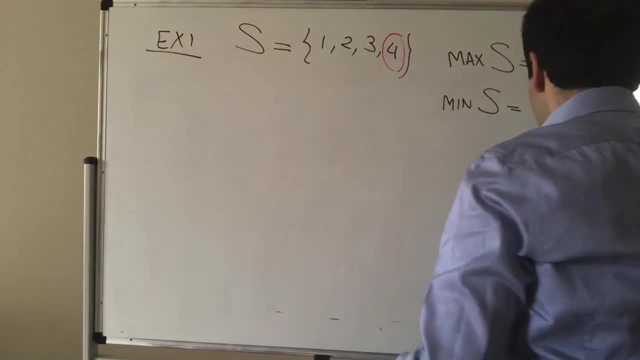 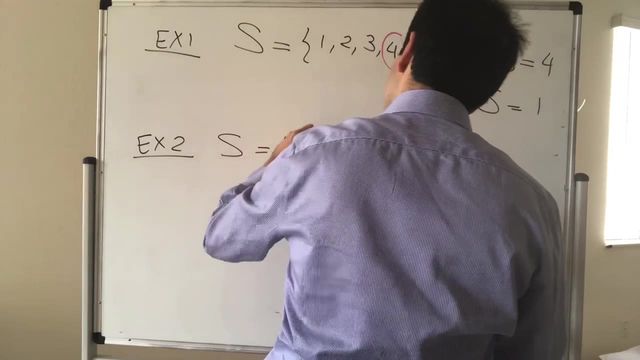 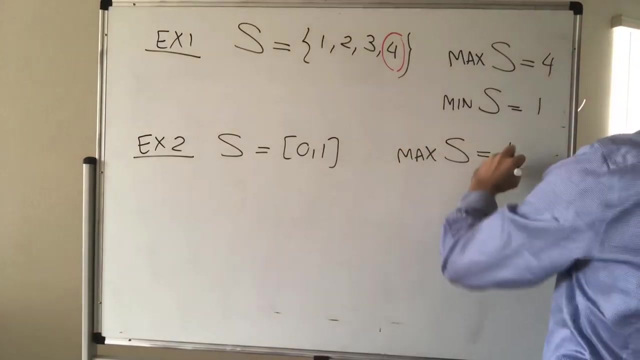 That's first of all. And then second example: again take S to be the interval zero comma one. Again this means closed interval. Then the maximum of S is one because again one is in your interval and it's bigger than all the other elements in that interval. 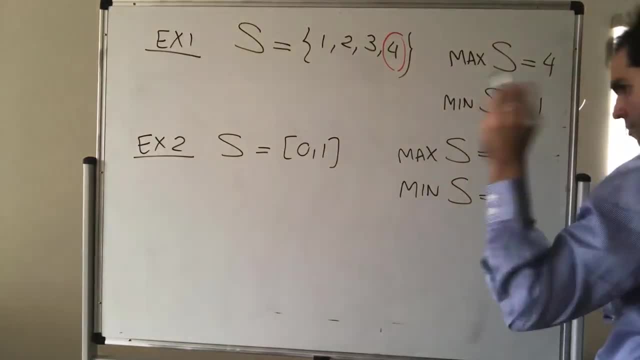 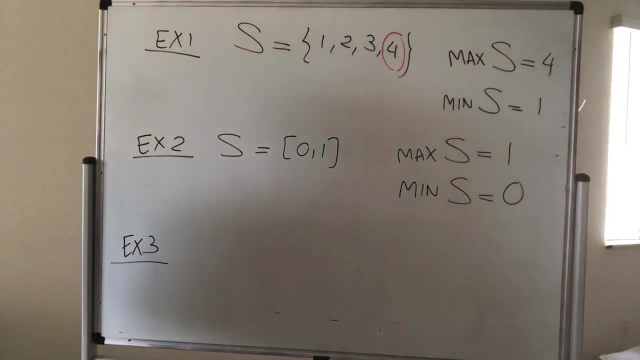 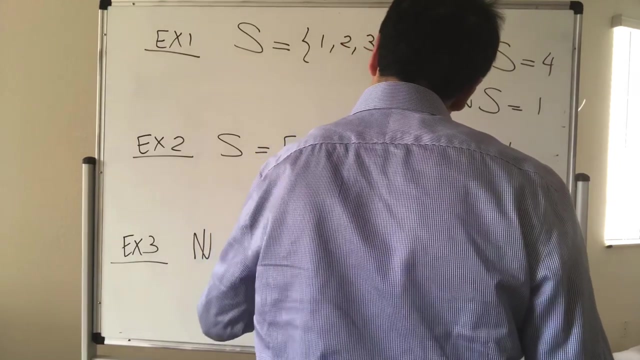 And the minimum of S is zero. Okay, well, how would a slightly more interesting example, take the natural numbers which, again remember, they start with one, one, two, three, dah, dah, dah. Then, yes, the natural numbers have a minimum. 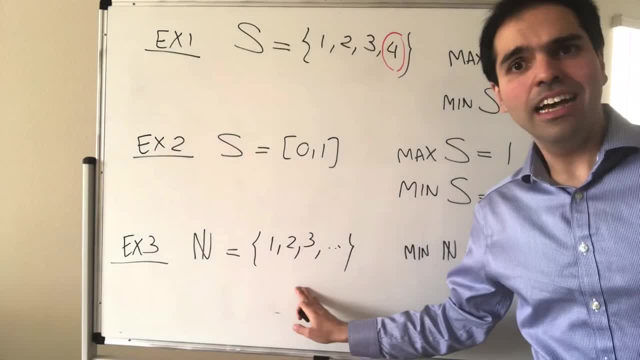 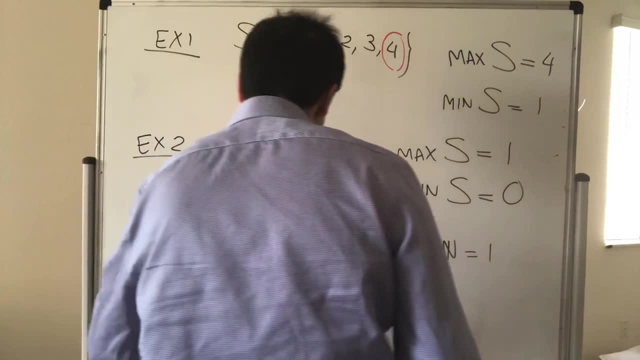 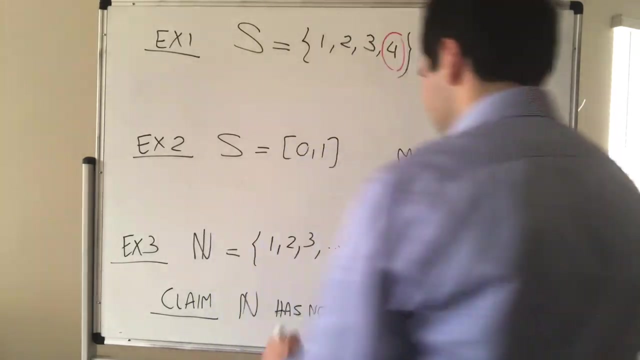 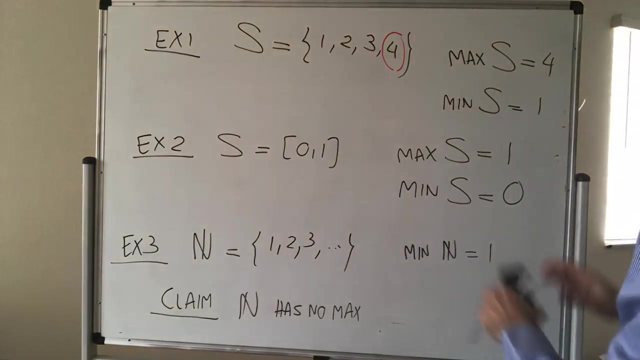 which is one. but I'm claiming that the natural numbers have no maximum. So claim N has no max and the maximum is zero. Intuitively it's clear, because N goes infinitely large, so it cannot have a biggest element. but the question is: how do we prove this? 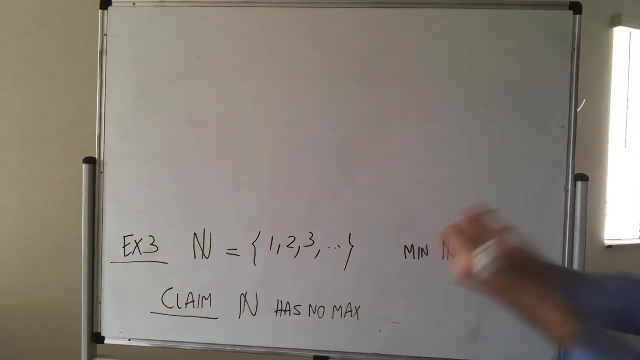 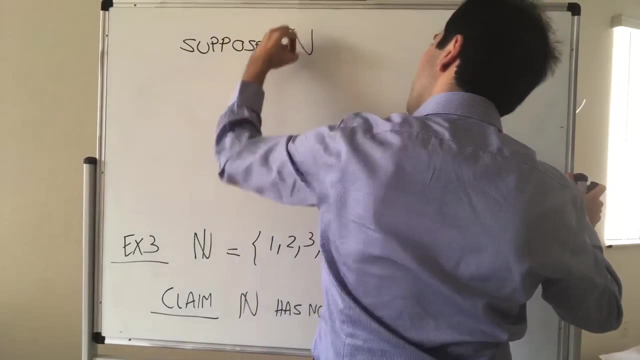 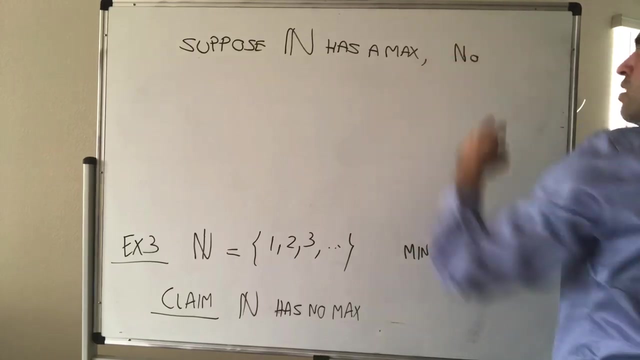 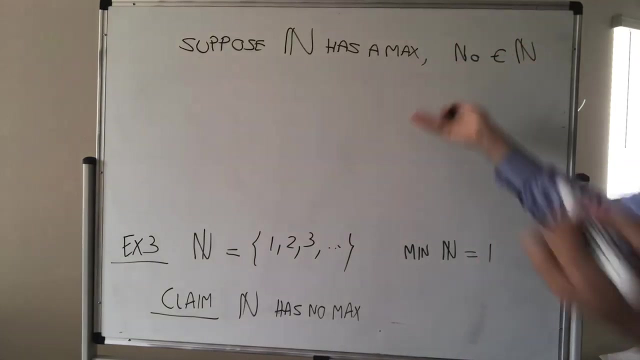 And the proof is very, very neat, because suppose N had a max, So suppose N has a max, Let's call this N naught. Then N? naught is an integer by definition, And also N naught is bigger than any other element in N. 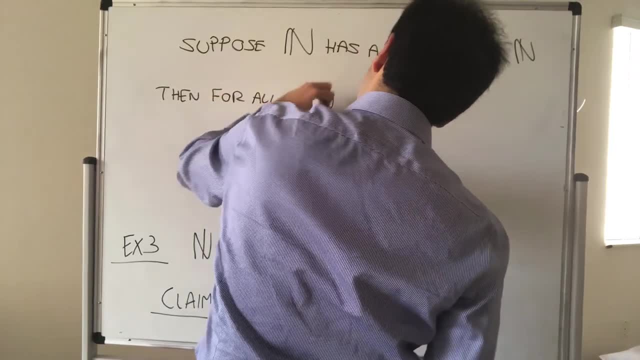 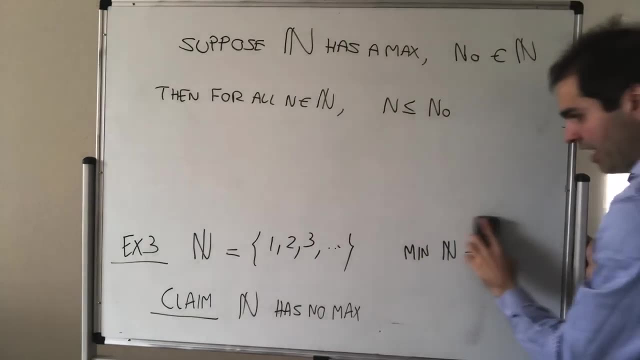 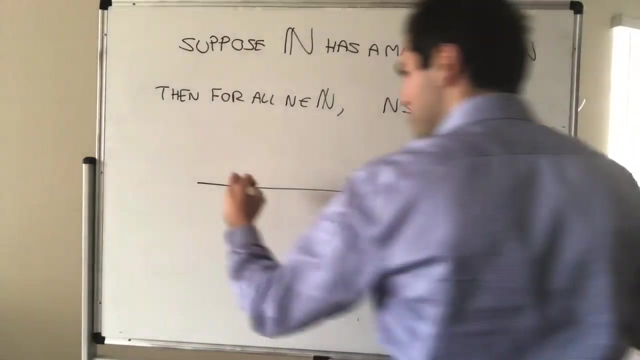 For all N. N is less than or equal to N, naught Again by definition of max And again very important, this holds for every natural number. So what I'm saying is, if this is N, one, two, three, et cetera, et cetera, 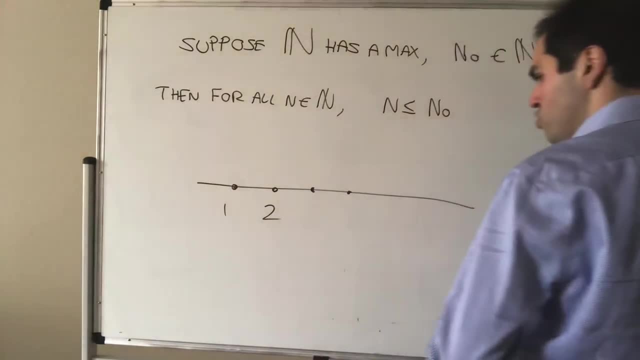 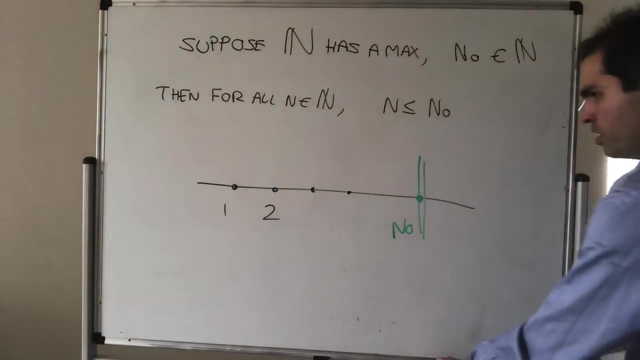 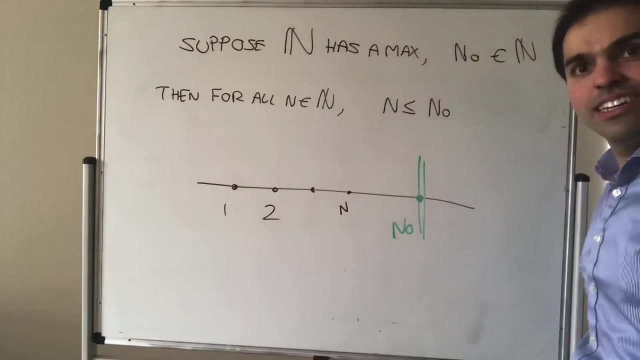 then this says that N naught is the biggest natural number there is. So this is N naught and there's nothing bigger than that. In other words, if you take a random natural number, it's smaller than N naught. But then can you give me a number that's bigger than N naught? 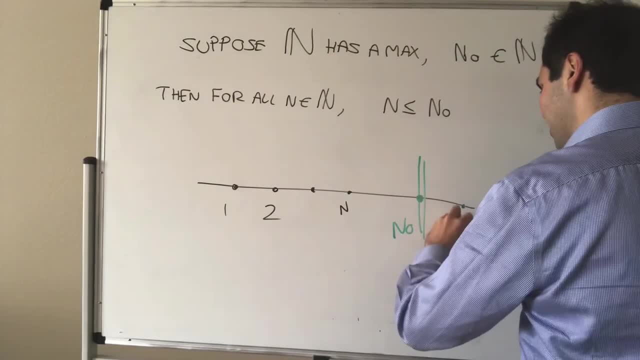 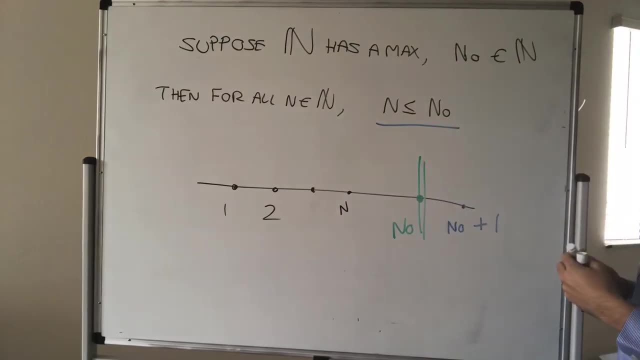 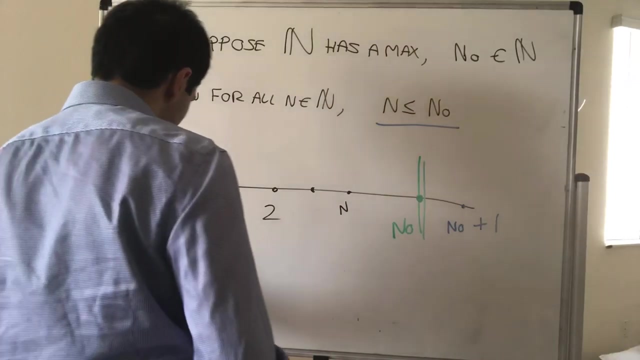 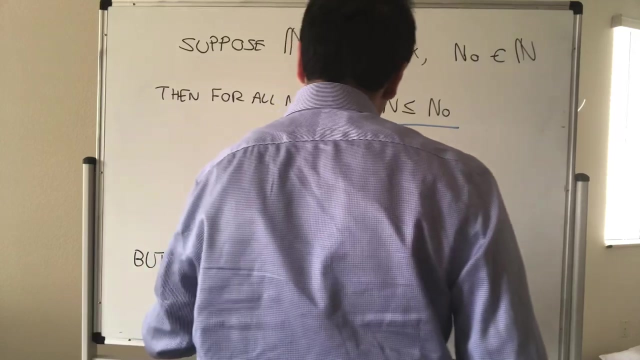 Why not, In other words, take N naught, N naught plus one. So you see, if this were true for every N, then it would also be true for N naught plus one. What now? Let N be N naught plus one. 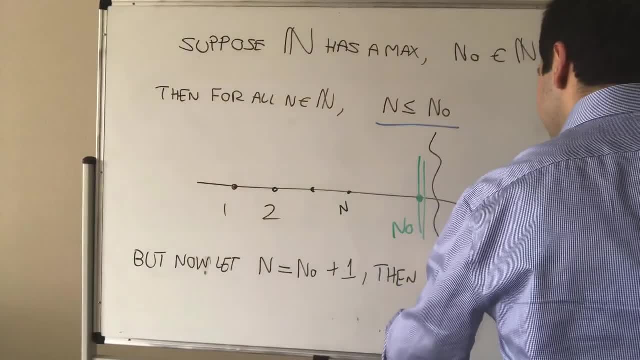 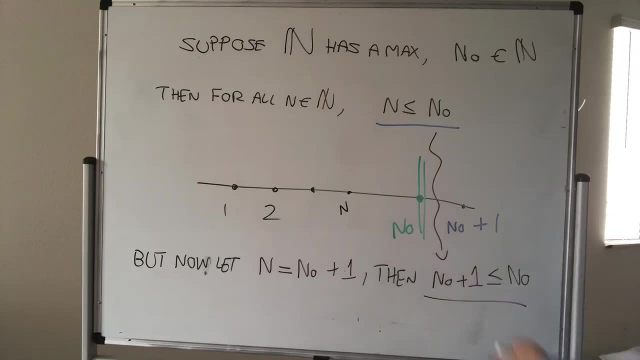 Then this thing: it's saying, indeed, that N naught plus one is less than or equal to N naught. But that's a contradiction. you know, The success of a number is not never smaller than or equal to the number itself. 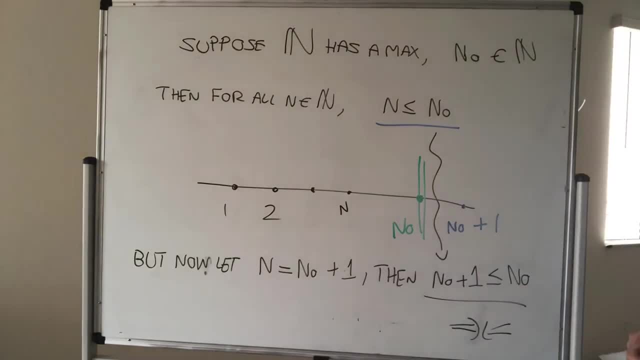 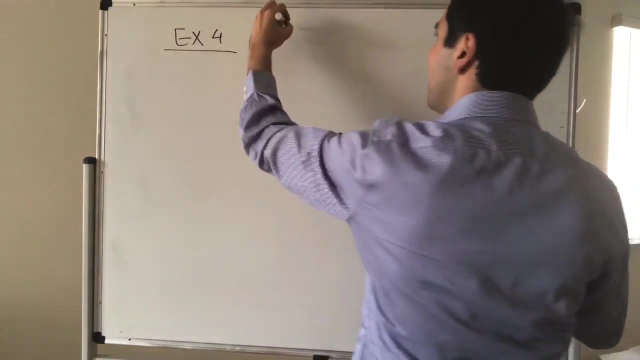 So it's a contradiction. A contradiction with what? A contradiction with the fact that N has a max, In other words, the natural numbers do not have a maximum. Here's a more interesting set set which, I have to admit, is a little bit more complicated. So let S be the set. 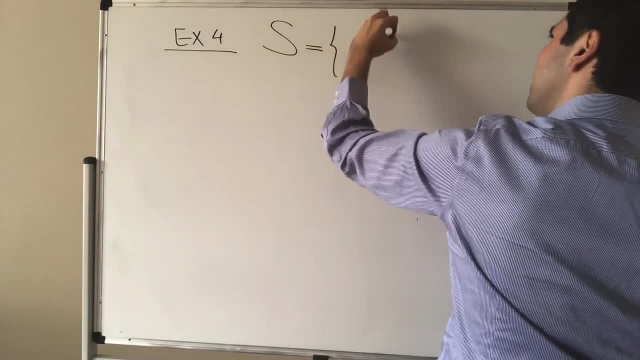 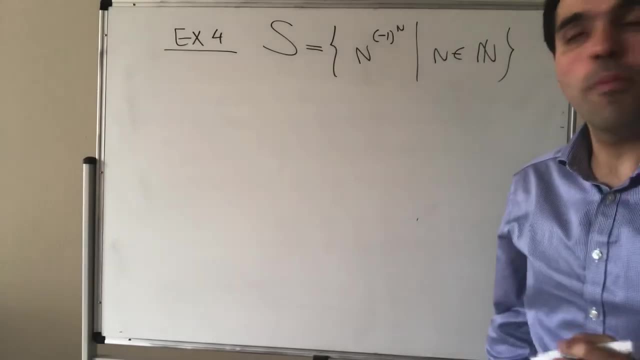 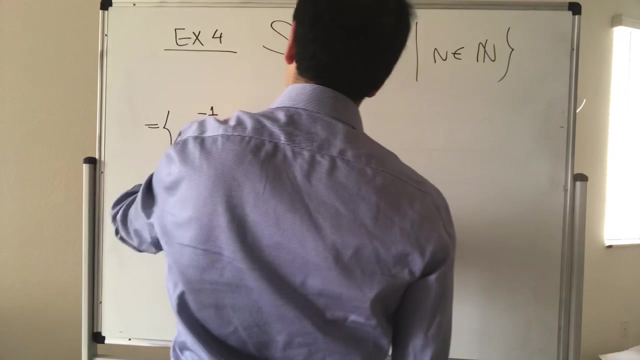 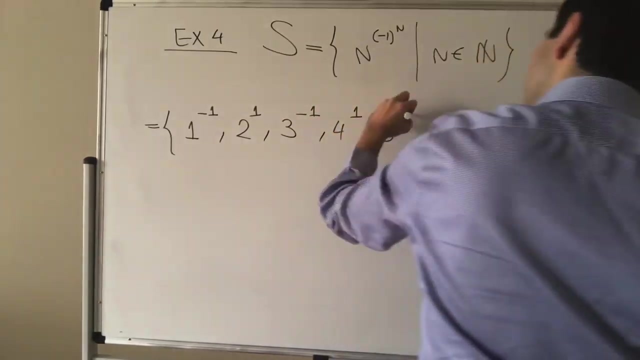 of the form n to the minus 1 to the n, where n is just an integer. So let's list a couple of examples. So this becomes, I think, 1 to the minus 1, and then 2 to the 1,, 3 to the minus 1, 4 to the 1,, 5 to the minus 1, 6 to the 1, etc. etc, And that's. 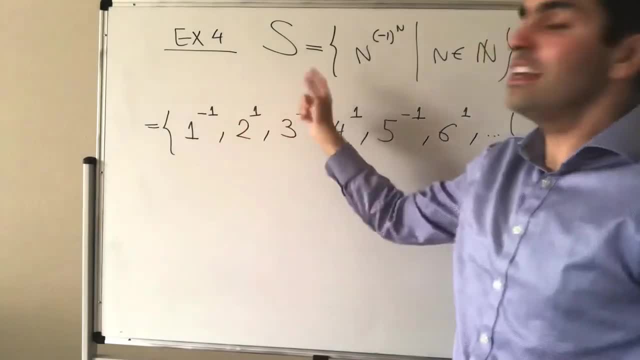 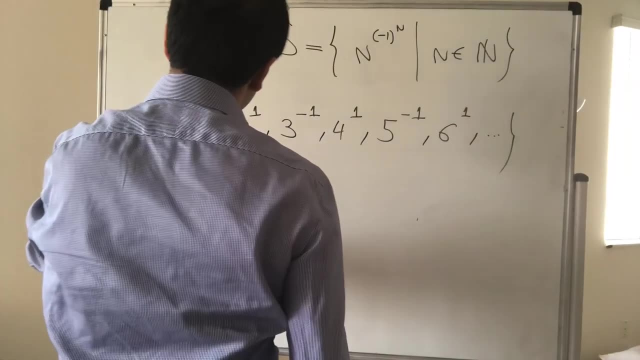 because minus 1 to the n alternates between minus 1 and 1.. So that's what this set is, and if you want this, just becomes 1, 2, 1 third, 4, 1 fifth, 6,, etc. 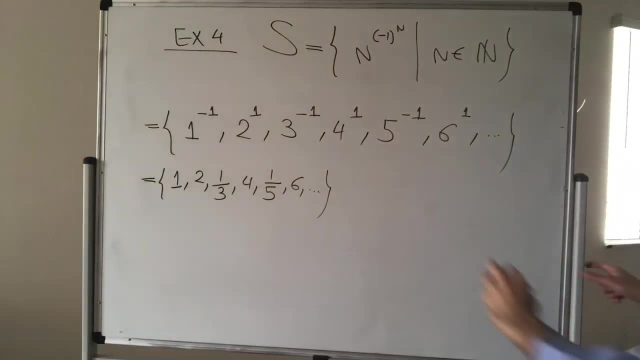 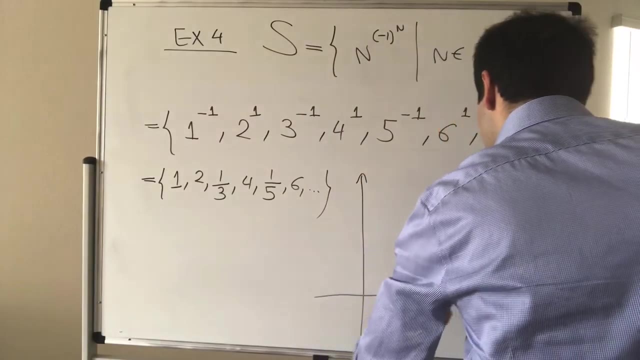 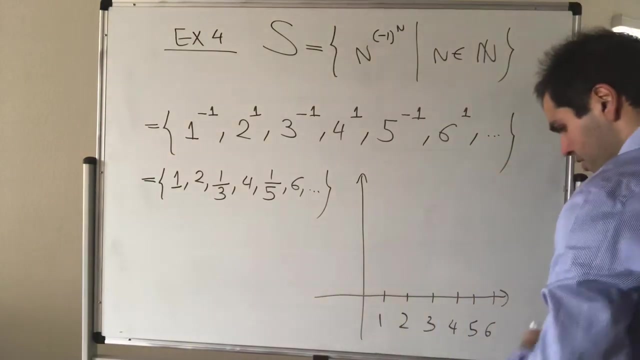 etc. So if you want to graph that out, what this becomes simply as follows: So this is 1,, 2,, 3,, 4,, 5, 6.. What's interesting to note is that the odd powers they go. 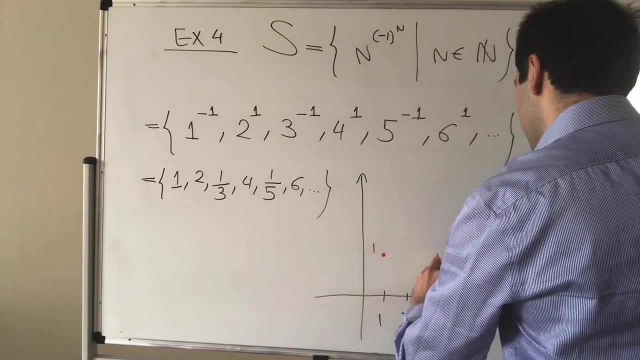 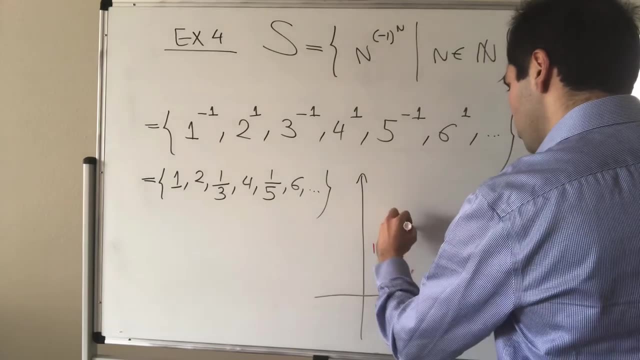 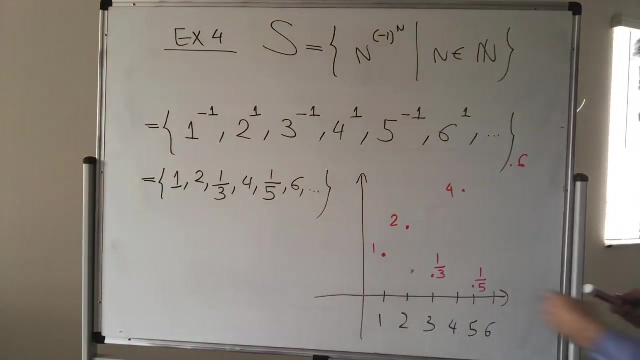 down, So 1,, 1 third, 1, fifth, but the even powers. they go up. So for instance, For instance, that's two and that's four, and that's six, And notice what is happening. In other words, the even powers. they grow without bounds. 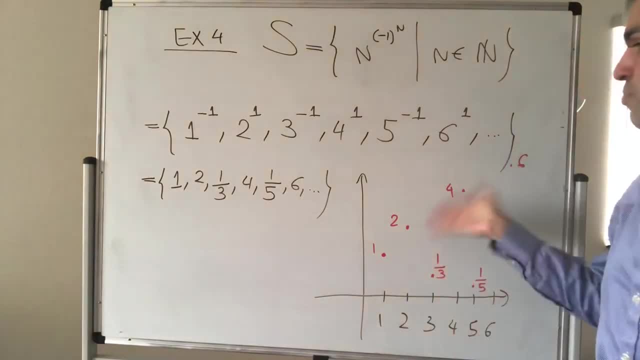 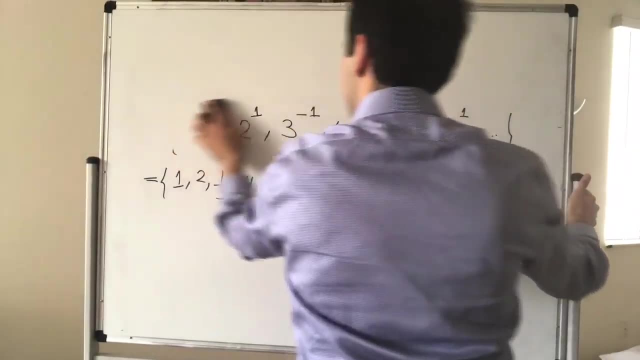 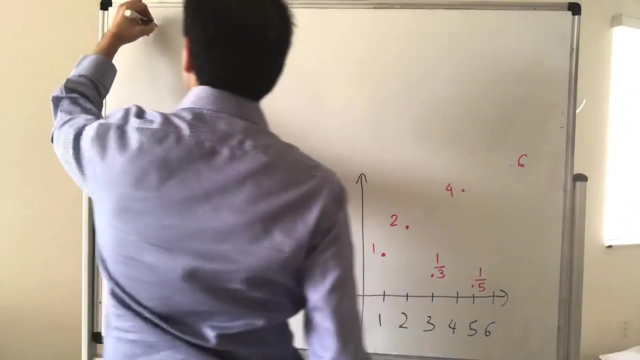 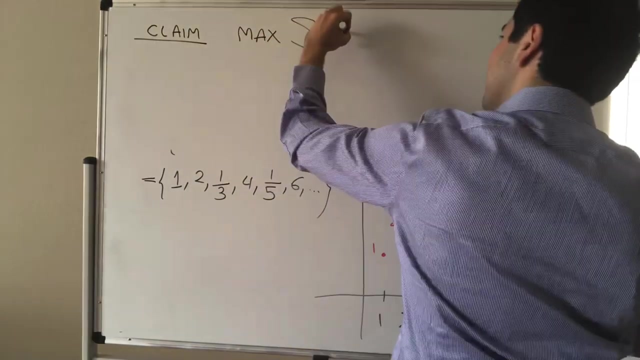 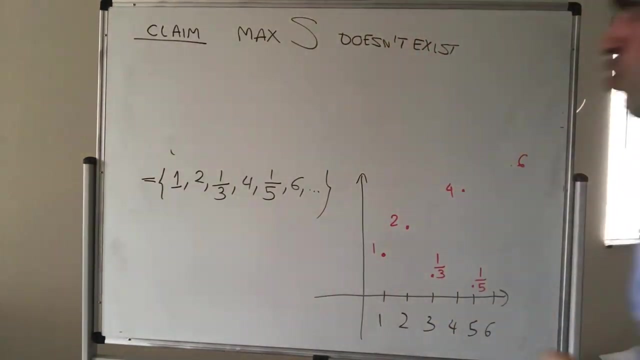 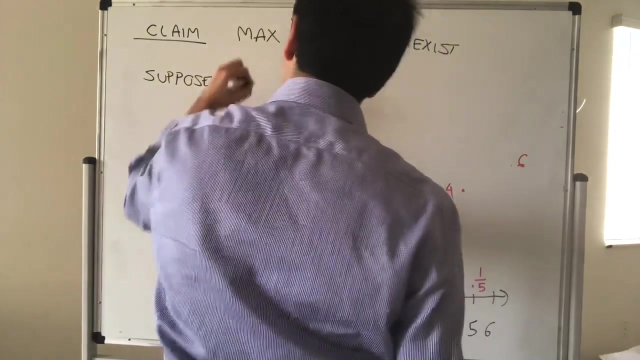 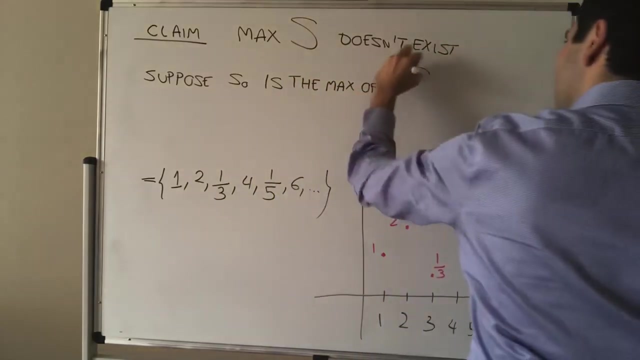 And in fact what I'm claiming is that the maximum of S doesn't exist. So claim Max S doesn't exist. So in other words, suppose S naught is the max of S Of S, Then essentially what this means? it means S naught isn't S. 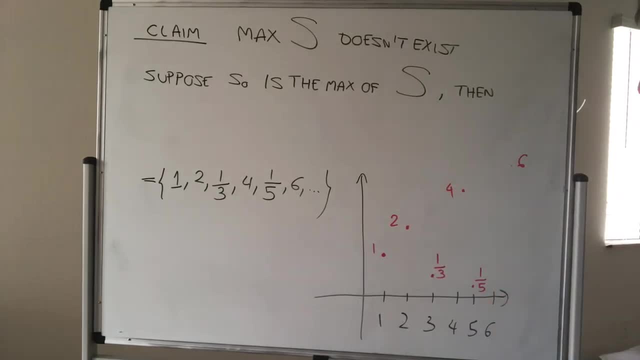 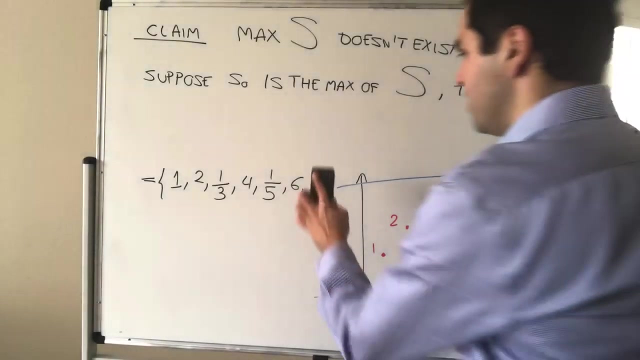 but, moreover, every element of S is smaller than S naught, So suppose I'm claiming: okay, this is the max of S Then, in other words, every values of S are smaller than this S naught And, equivalently, all that this means is that 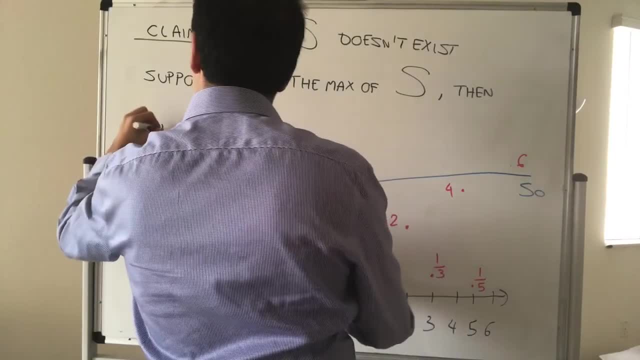 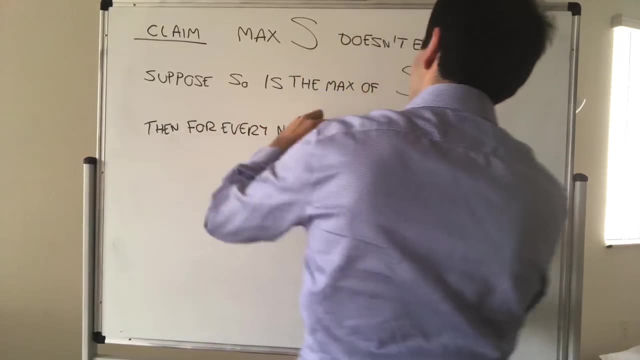 for every n. what this is is that every n is equal to, equal to S naught for every n. for every n is equal to S naught, the sum of all is equal to n, n, n. 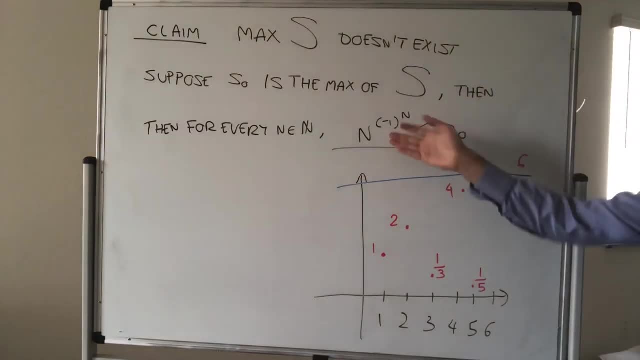 We have that n to the minus, one to the n is less than or equal to S naught. In other words, a generic element of S has to be less than or equal to S naught. But again, notice what is happening. 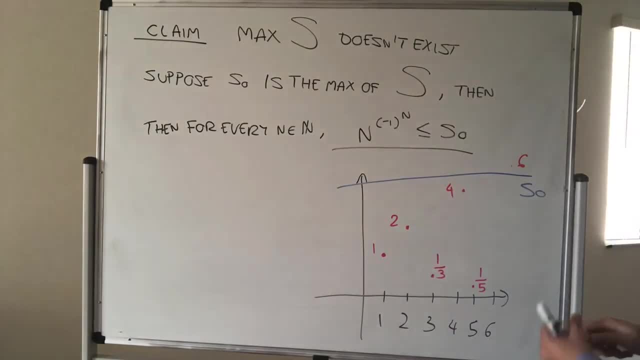 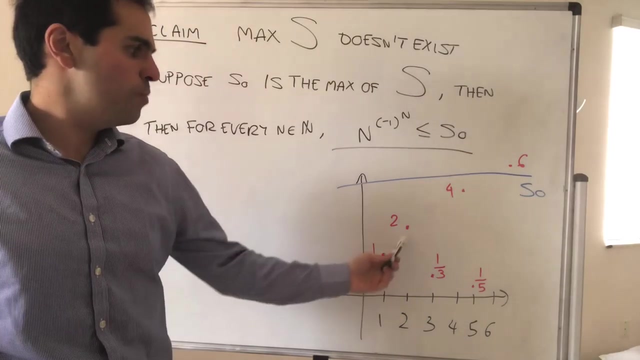 the even, powers grow without bounds. So essentially, here's the idea: what we want to choose is is simply an even number that is bigger than s naught, because that way we can go above s naught. but again, we have to choose even numbers because notice the 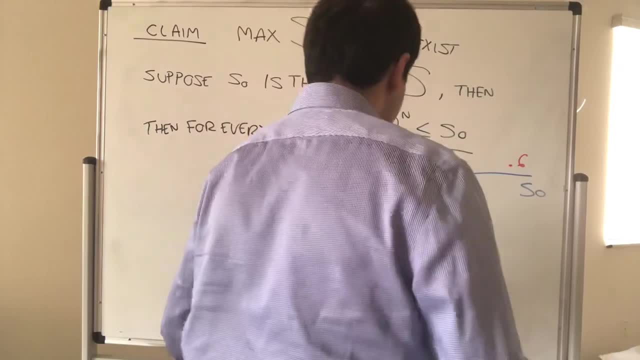 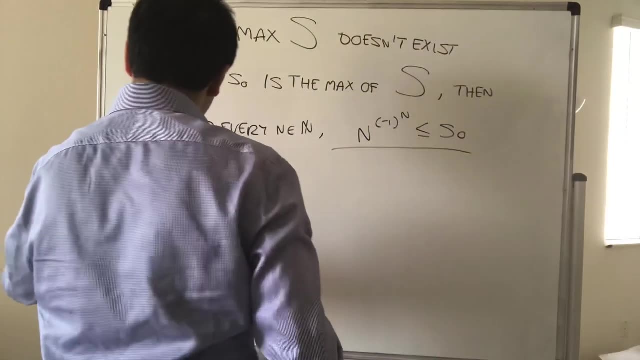 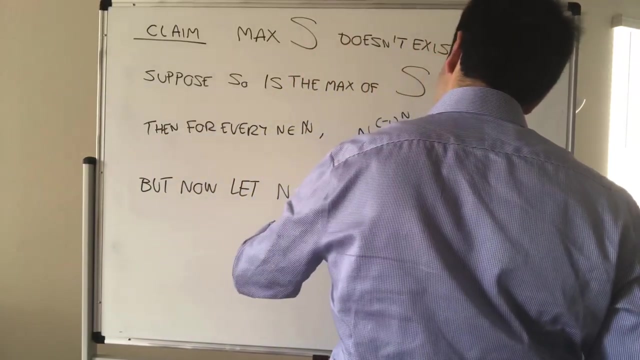 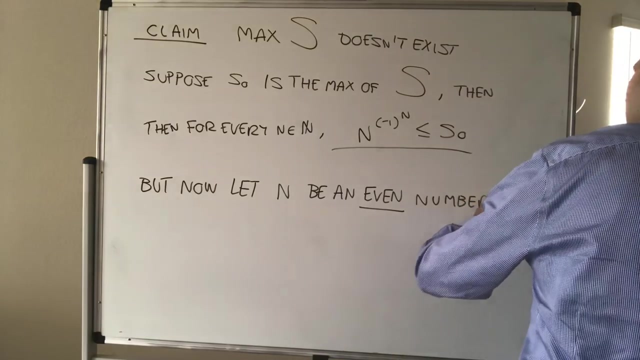 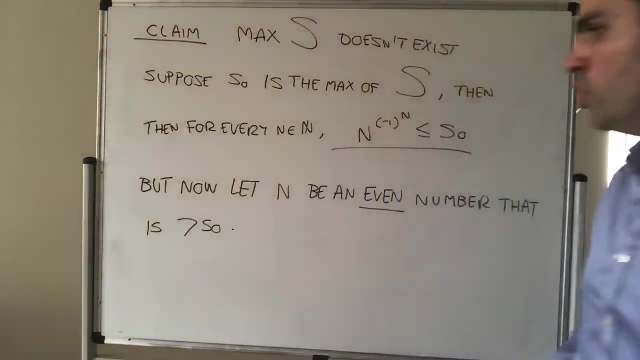 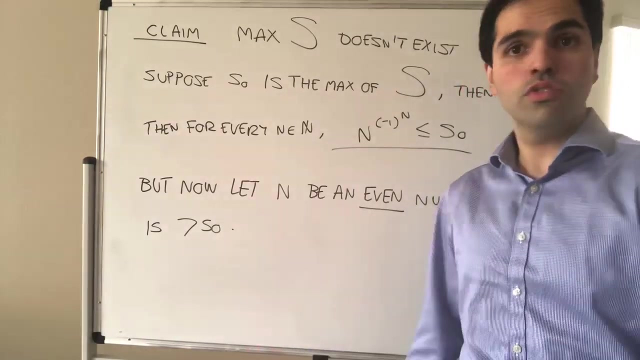 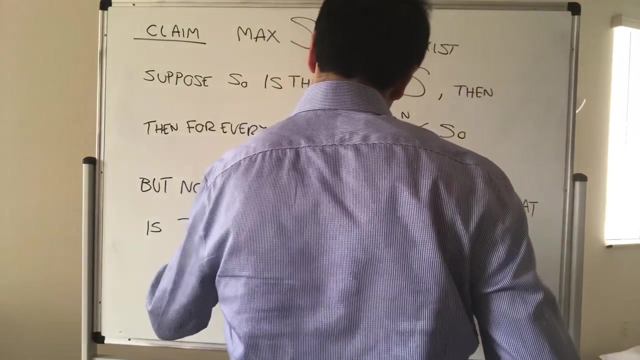 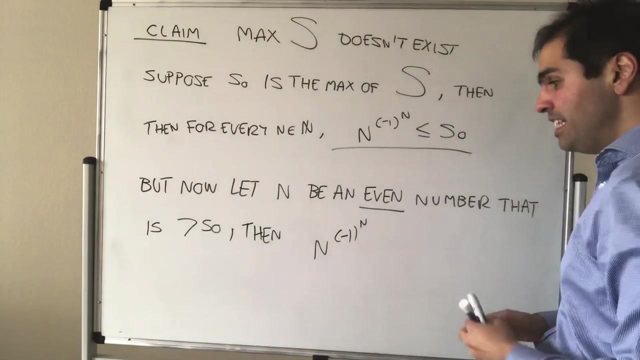 odd powers they go down. so in other words, simply that that is strictly greater than s naught. so again, if i told you s naught is 9001, just choose 9002. if s naught is 22, just choose 24. okay, then, what do we have? well, n to the minus, 1 to the n. remember, n is an even number here. 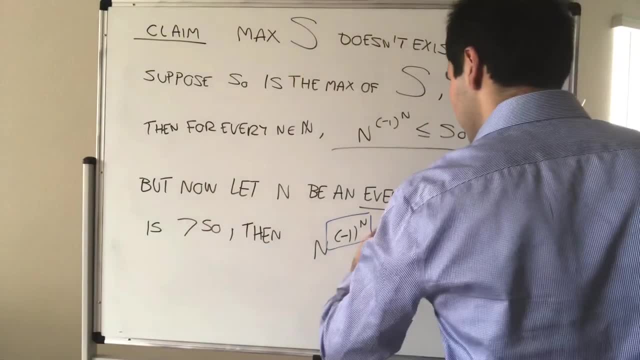 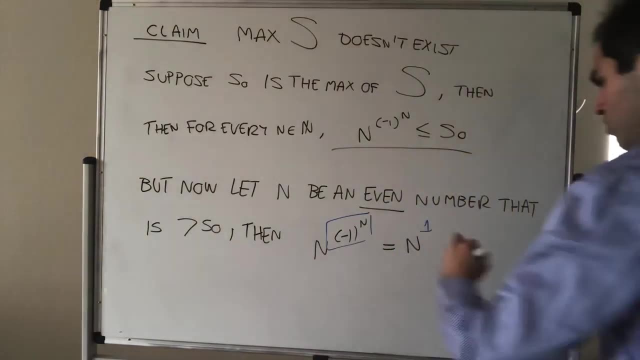 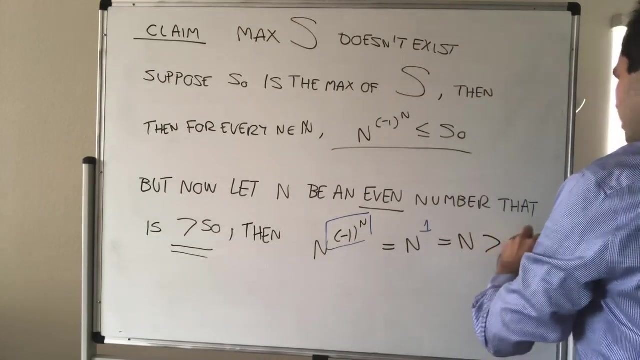 so minus 1 to the n just becomes 1. so that becomes n to the 1. so but n to the 1 is just n and by assumption, by your selection for of n, we know that this is greater than s naught. but then we have a contradiction, because on the one hand n to 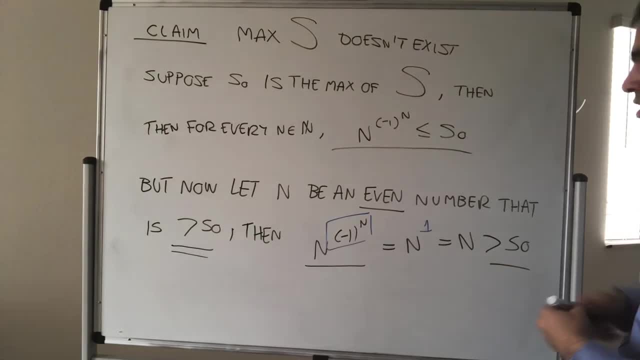 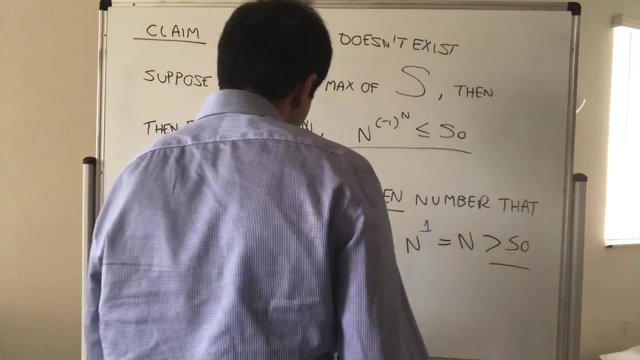 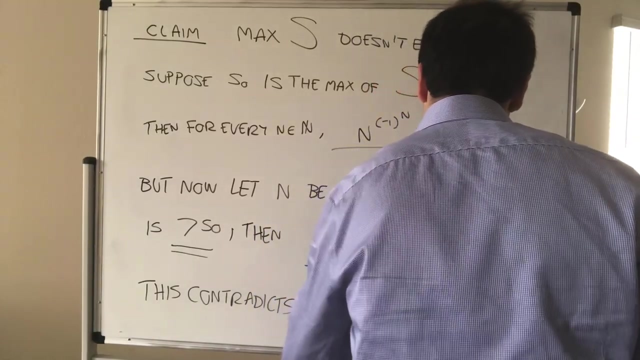 the minus 1 to the n is greater than s naught. but we also know that, no matter what n is, n to the minus 1 to the n is less than or equal to s naught. so we have a contradiction. so this contradicts: n to the minus 1 to the n is less than or equal to s naught. contradiction with what contradiction? 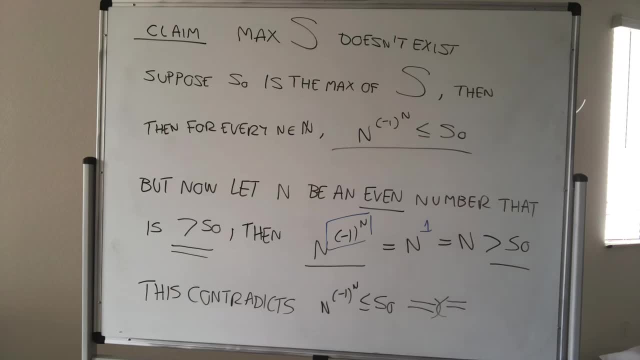 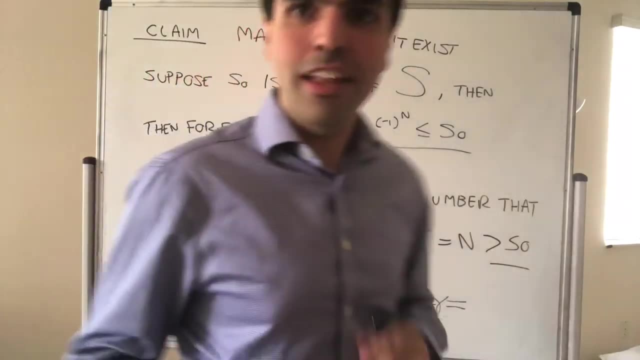 with the fact that s has a maximum and also- interestingly, we'll see- s also doesn't have a minimum, but we'll talk about that in one of the other videos. so thank you so much for watching and i'll see you next time. bye, bye, bye. 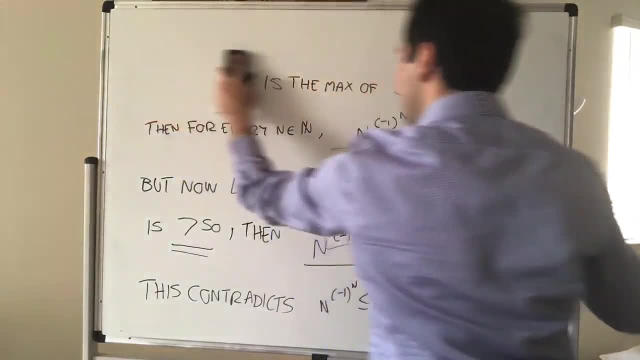 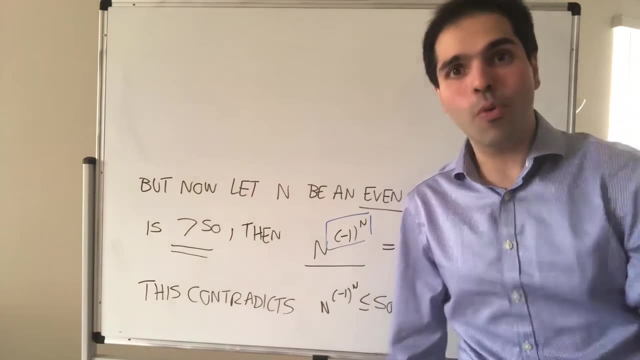 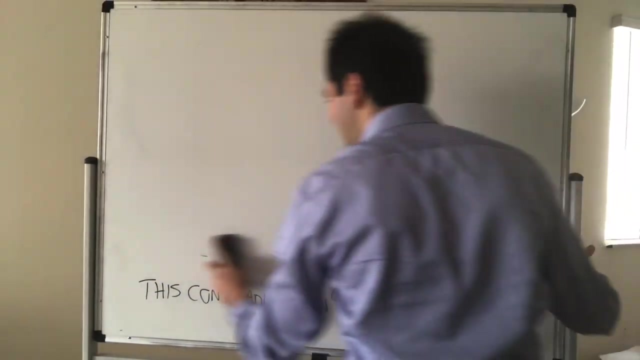 the next videos. Okay, very good. Last but not least, I wanna emphasize: it's very important that your maximum be in your set, So your maximum has to be an S and, in fact, the following: it's an amazing illustration of that fact. 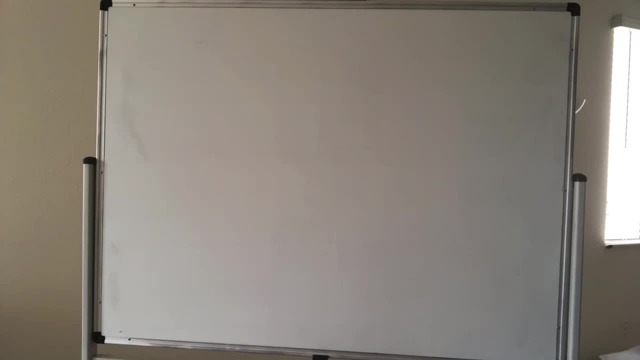 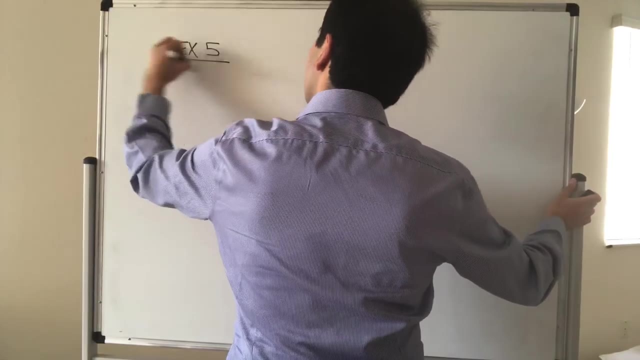 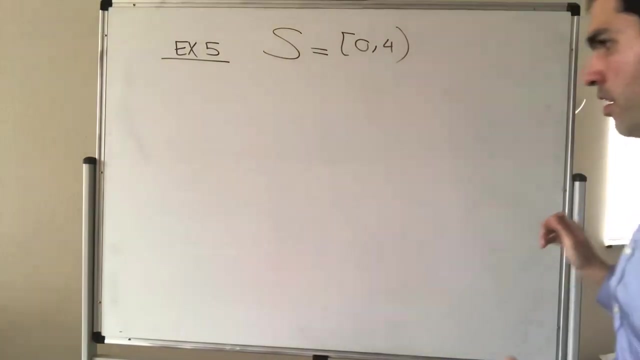 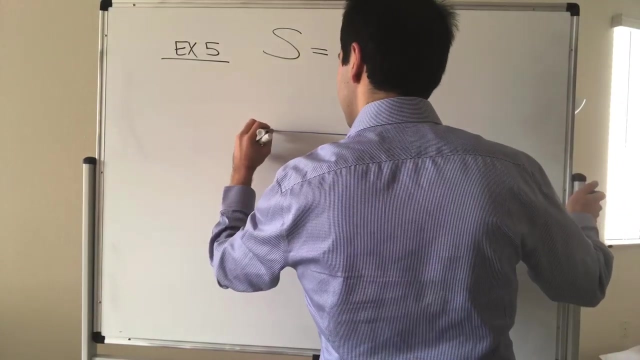 So I don't know why I wrote example four. that was well, I guess, example five. now, Okay, Consider the following: So S is the set zero comma four. okay, So again, just the interval zero comma four. So it includes zero, but it does not include four. 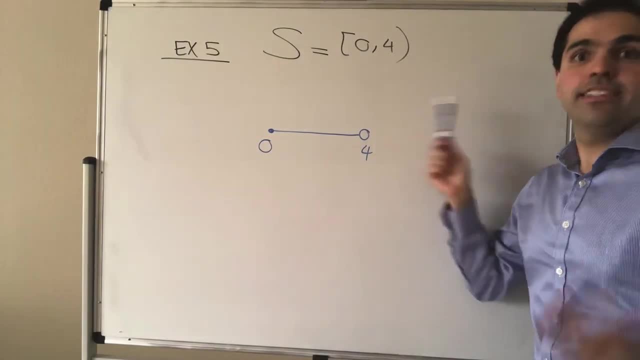 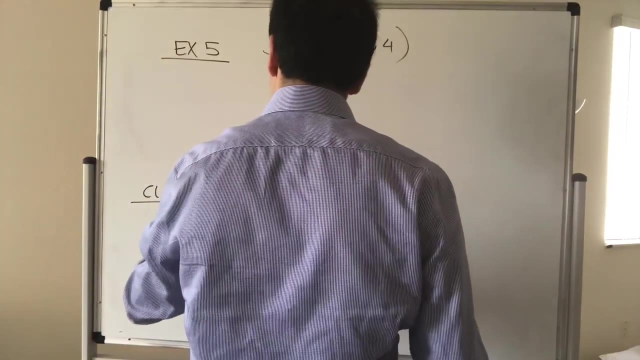 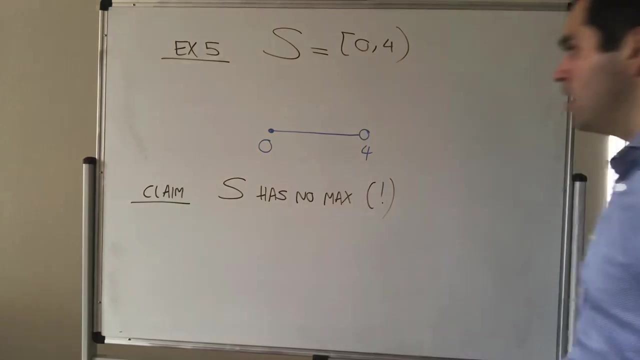 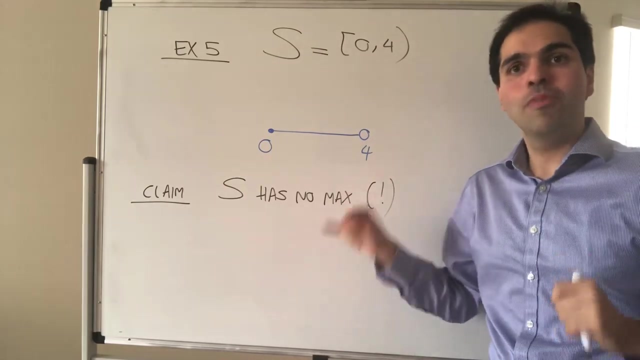 And indeed I'm claiming that this set has no maximum. Okay, Claim S has no max. In fact it's interesting because you would think four is the maximum. but remember, by definition the maximum has to be in your set. 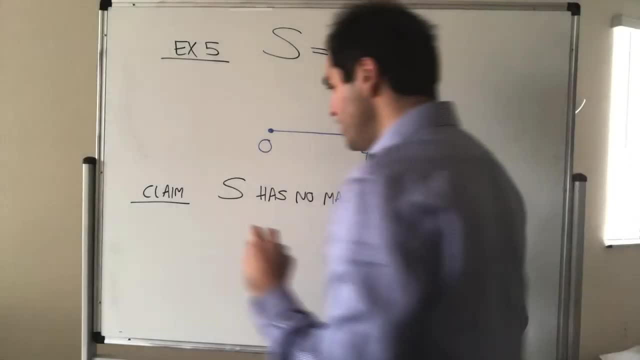 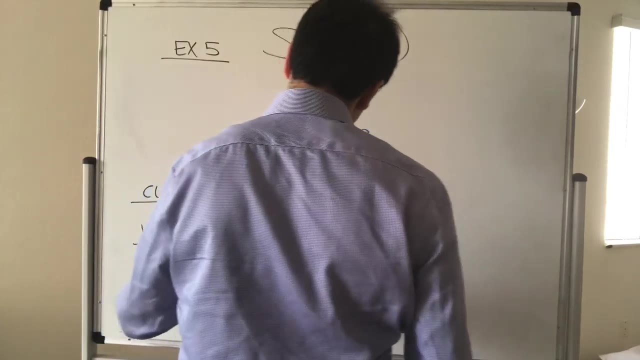 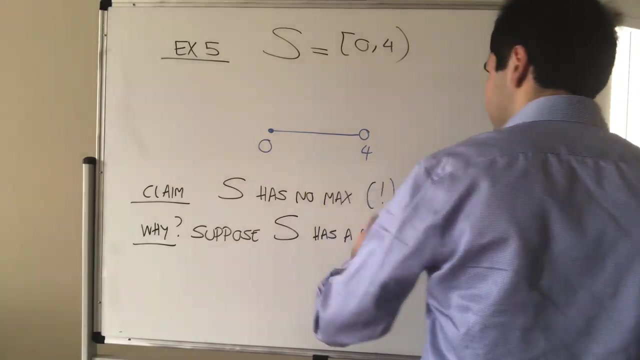 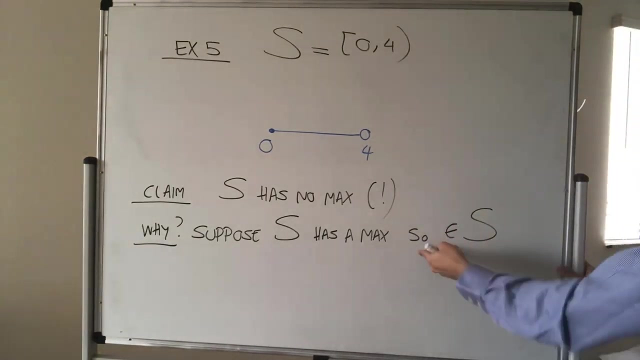 So four cannot be the maximum. And here's why, Suppose S had a maximum, Let's call it S naught. S naught, by definition, is in your interval. So in particular, S naught, by definition, has to be strictly less than four. 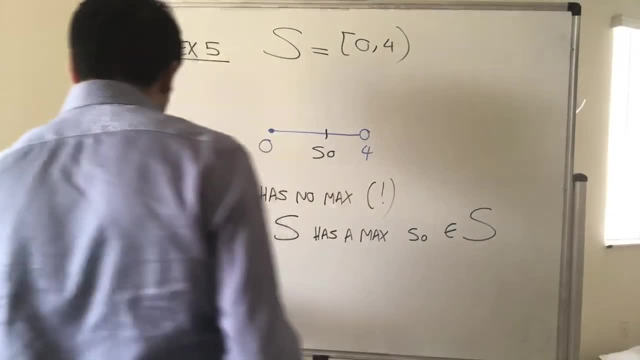 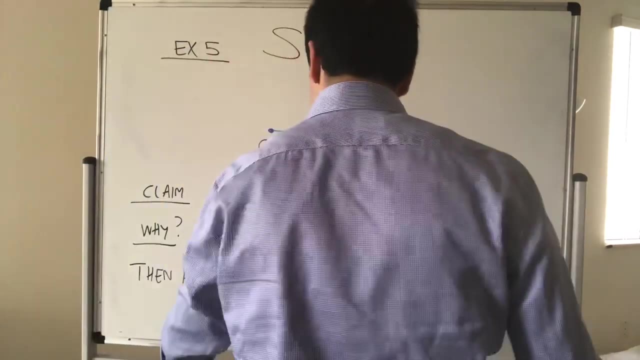 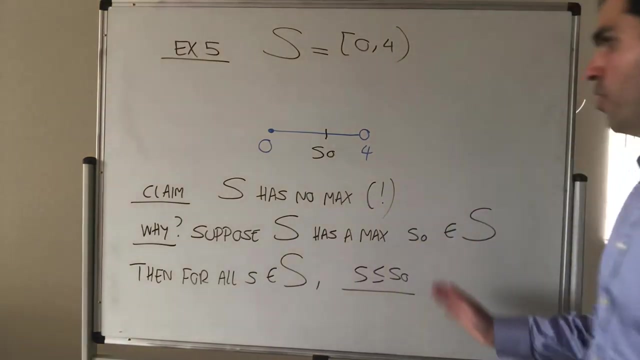 So S naught might be in there. So then, for all S, we know that S has to be less than or equal to S naught, So any element in S has to be less than or equal to S naught. But that's a problem, because how about we let S? 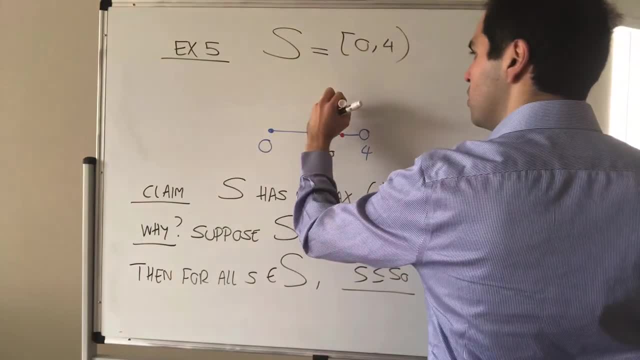 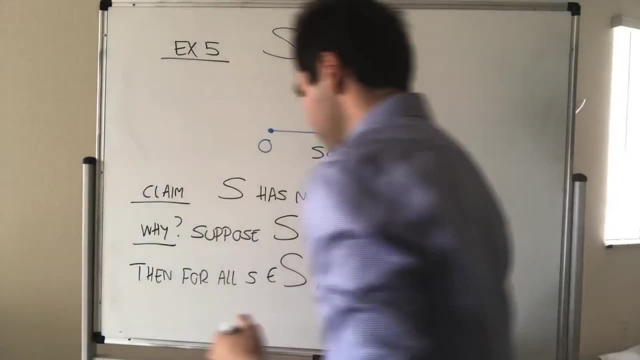 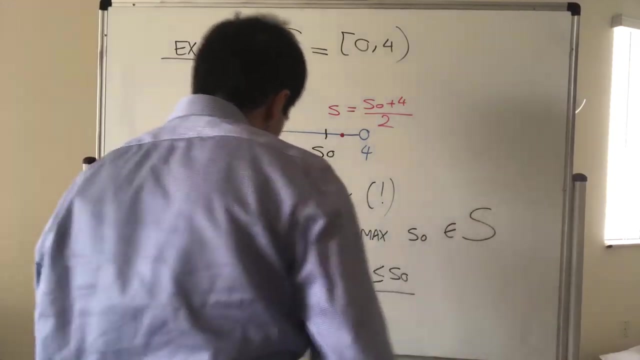 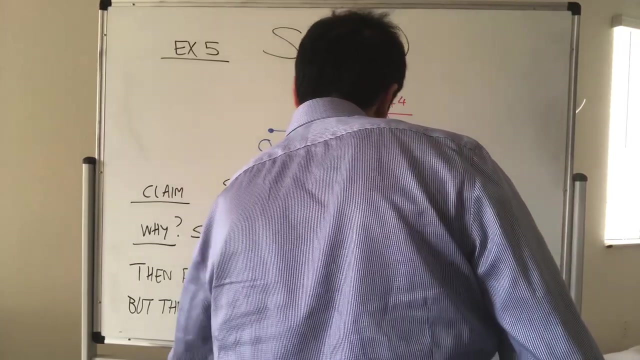 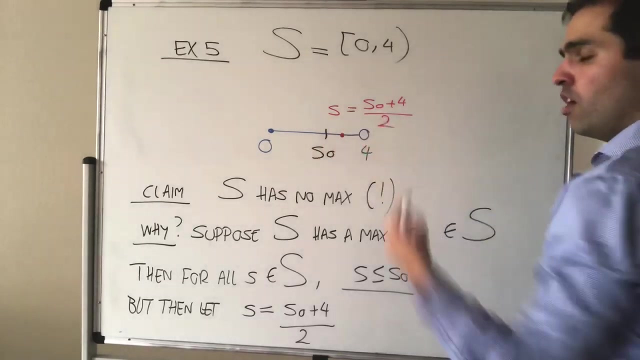 be the following, just to be the midpoint between the two. So let S just be the midpoint. Let S be again S naught plus four over two, And again, because it's the midpoint, it has to be strictly less than four. 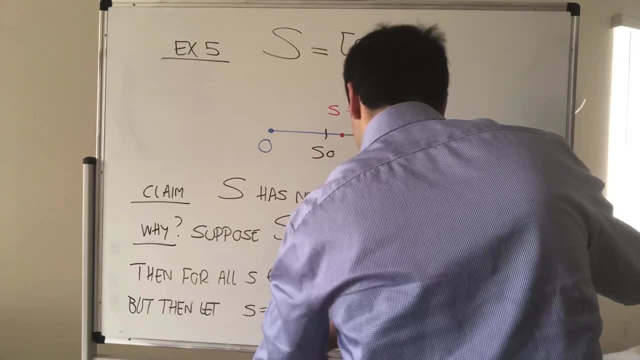 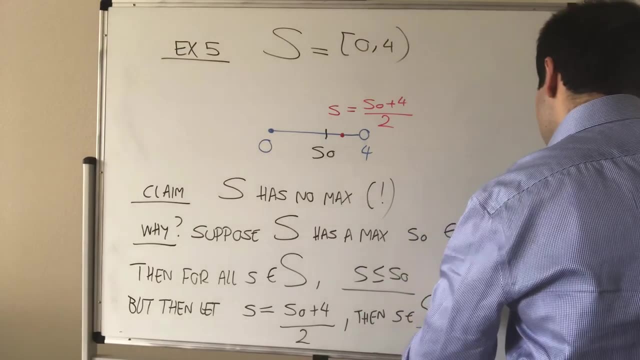 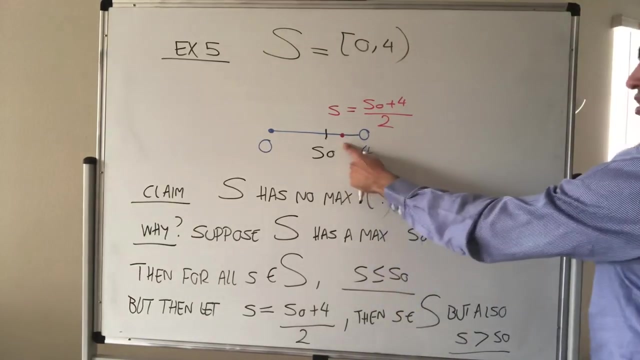 but also strictly greater than S naught. Then again S is an S, again by construction, but also S is strictly greater than S naught, Again by construction, because it's the midpoint of the two points. But then we get another contradiction. 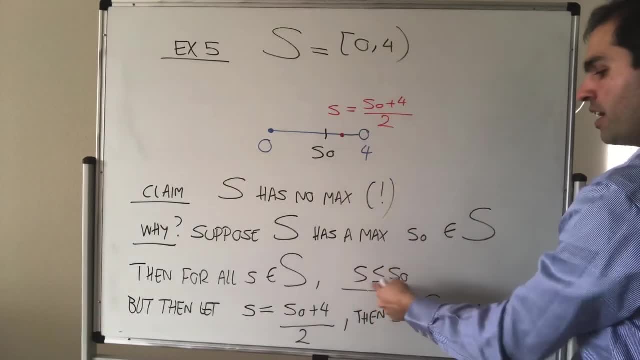 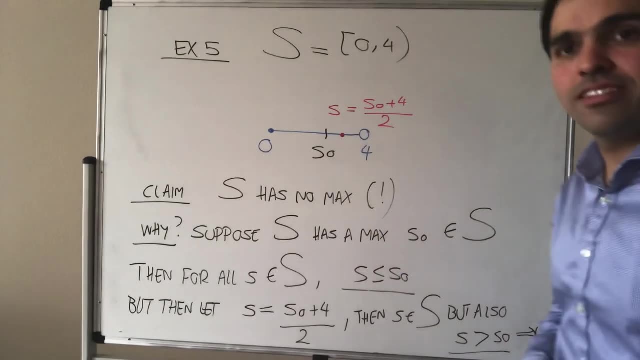 Because we assume that, no matter which element you pick, it's less than or equal to S naught by maximum S, But we also shown that this specific S is greater than S naught And that's a contradiction and in fact, 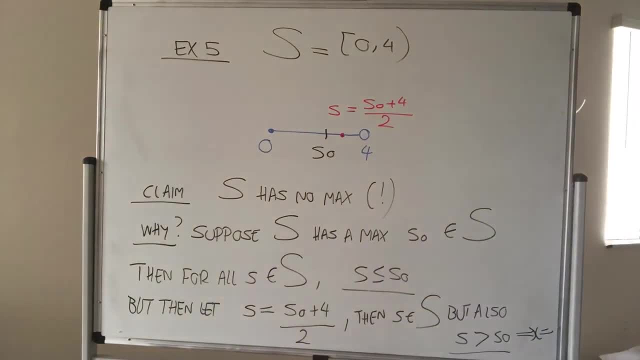 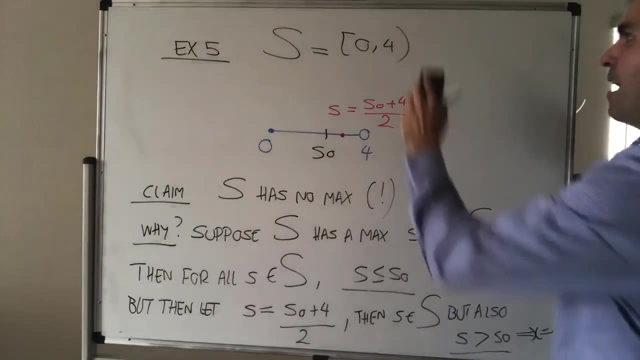 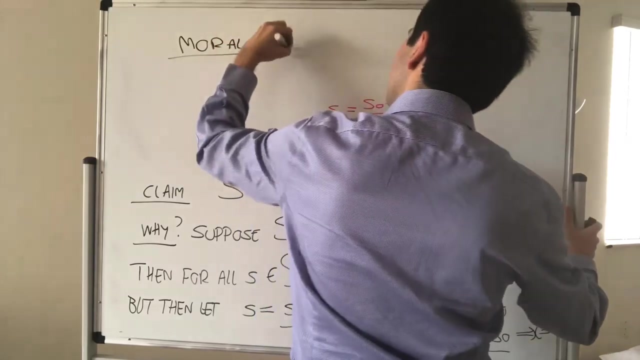 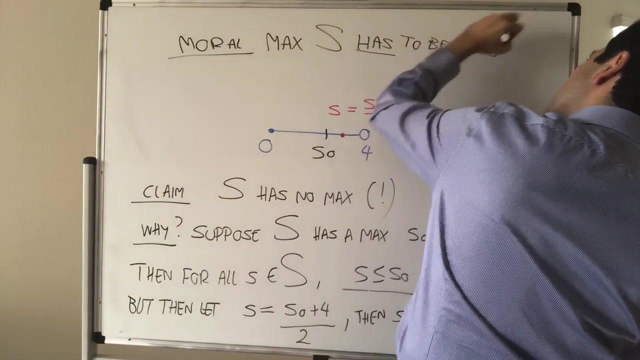 it shows that S has no maximum. So again, what is the moral of this story? The moral is: your maximum has to be in your set, So max of S has to be S. But I don't know if this bothers you. 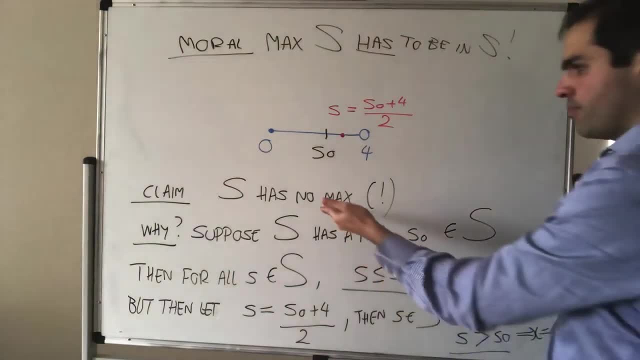 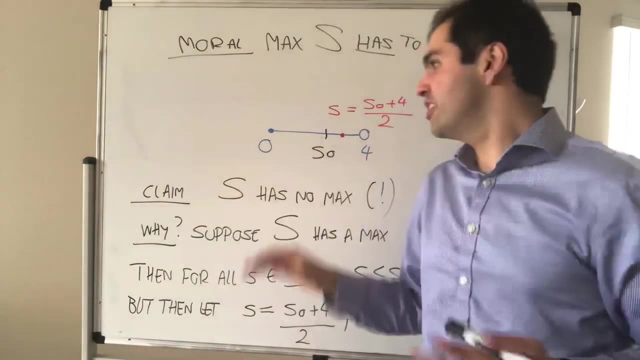 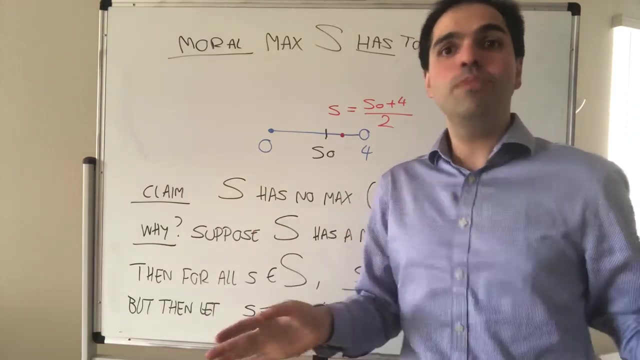 It really bothers me at least, because You see, intuitively speaking, four should be the maximum. I mean it is bigger than all the other elements in your set. but the only thing that sort of makes it not be the maximum is because in our definition of maximum